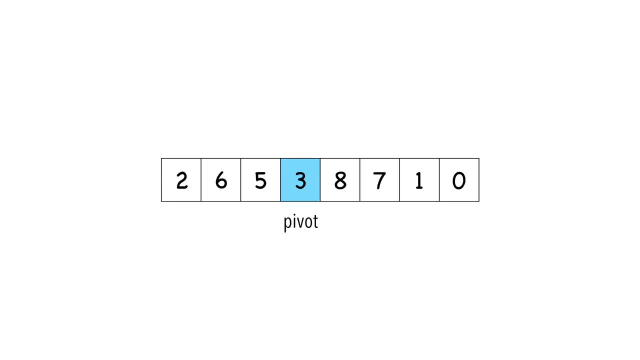 but for now let's just choose three. First, we move the pivot to the end of the array to get it out of our way. Next, we're going to look for two items: Item from left, which is the first item starting from the left that is larger than our pivot. Second, item from right, which is 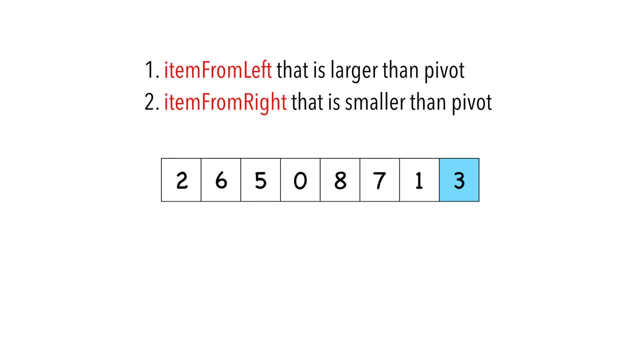 the first item starting from the right that is smaller than our pivot. Starting at two, we can see that six is item from left. Now, starting at the right, we see that one is item from right. Let's swap item from left with item from right. 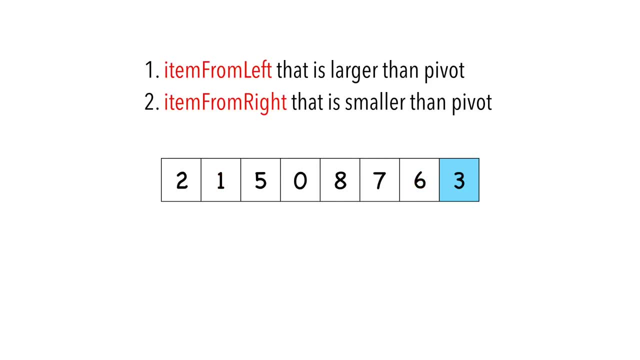 We repeat the process. This time, five is item from left and zero is item from right. Again, we swap the two One more time. This time we see that item from left has a greater index than item from right. so we know we're done. 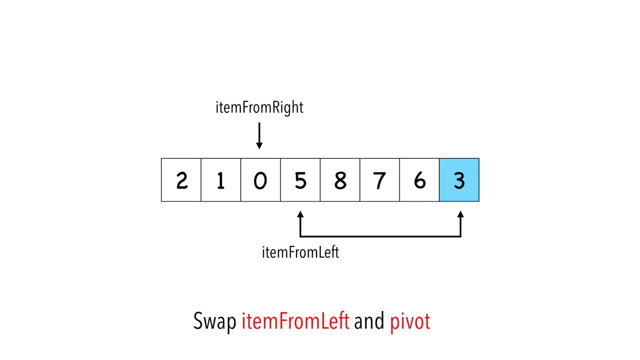 We swap item from left with our pivot Three. our pivot is now in its correct spot. To prove it, let's review our three conditions. As you can see, all items to the left are smaller and all items to the right are larger. 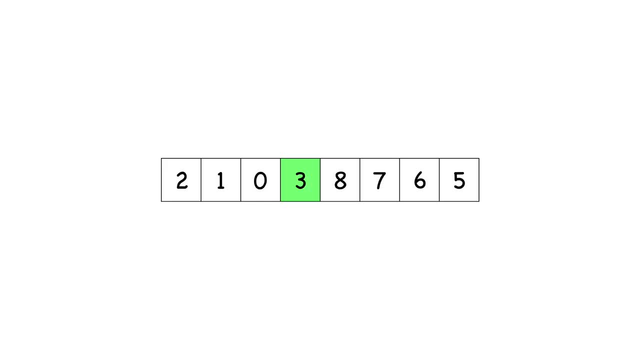 We said quicksort is recursive. Let's go through the process one more time. You can see how it works with a larger partition we just made. We'll choose seven as our pivot and move it to the end. I'll let you watch without voiceover. 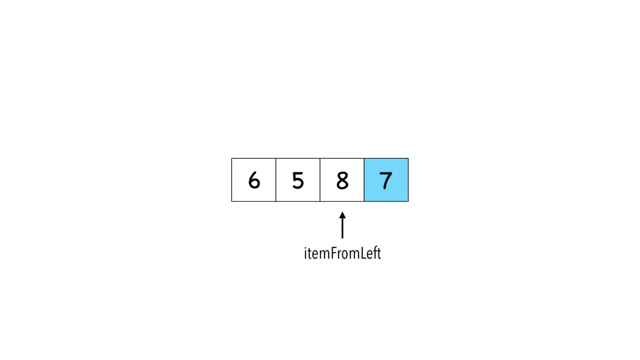 Now we have 3 and 7 in their correct positions. I think you understand the concept, so we'll let recursion handle the rest. One important question is how do we choose the pivot? This makes a large difference in the performance of the algorithm, as we want to choose a pivot.